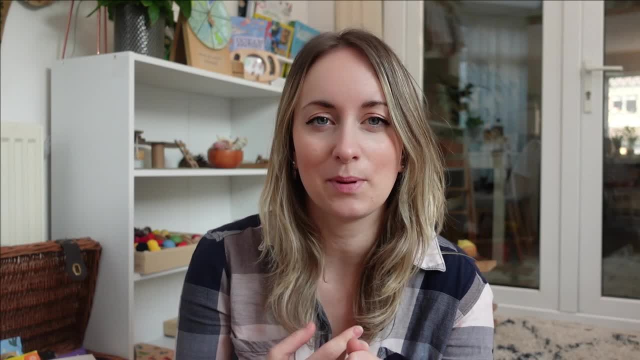 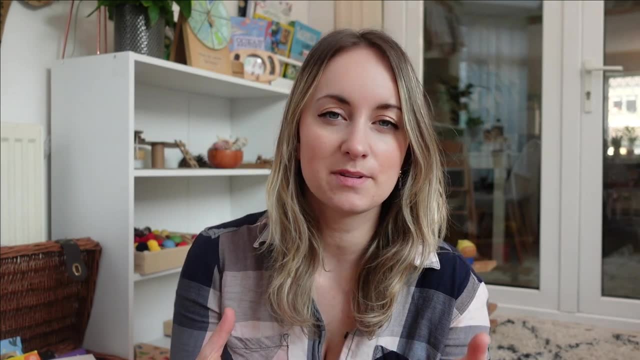 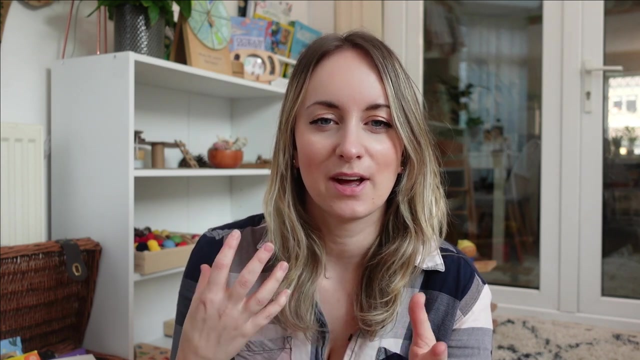 lots of can be such random objects, random pieces, But it's just kind of an area for a child to go to and explore And you're provided materials that will invite them to explore. So really interesting things. things are tangible, things that could spark a conversation or an. 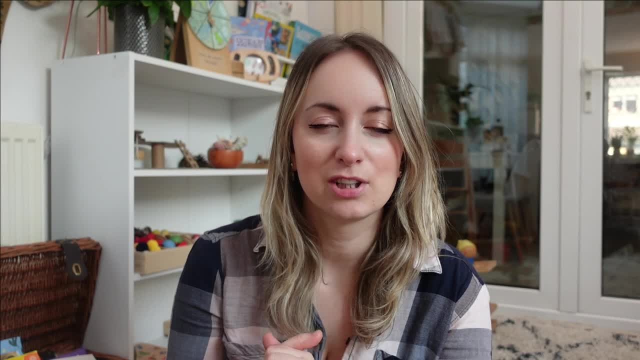 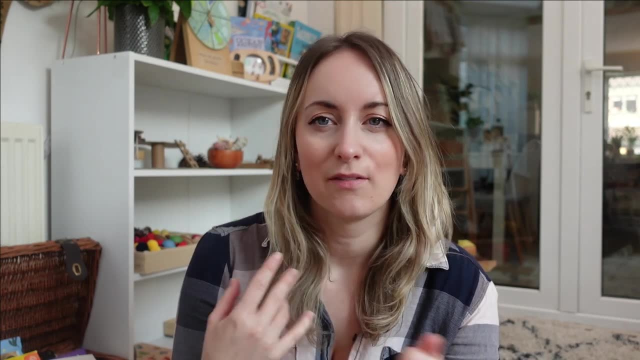 interest And there's so many different variations And they're always open ended materials, So always things that can be used in so many different ways. So here's an example: Shells are open ended. They can be used for sorting by size. 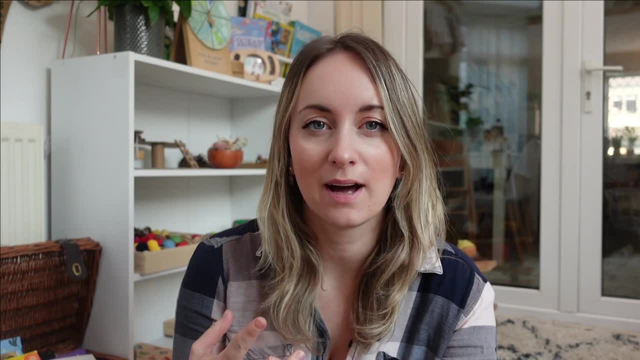 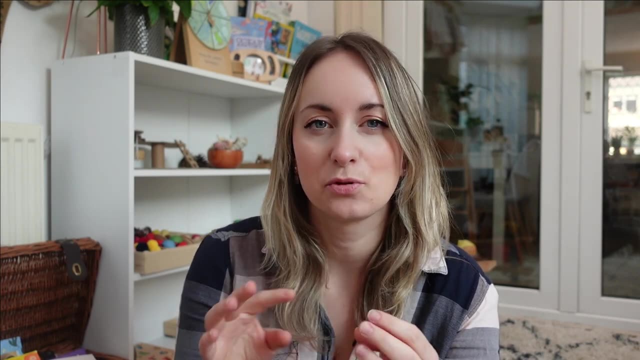 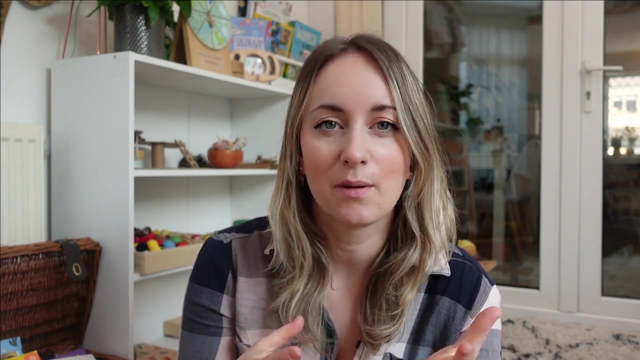 They could be used for counting and sorting by colour. It could be a sensory thing. You can feel all the different textures of shells and you can smell them. You can talk about shapes. There's- yeah, I mean lining them up- There's so many different options. You can fill them children. 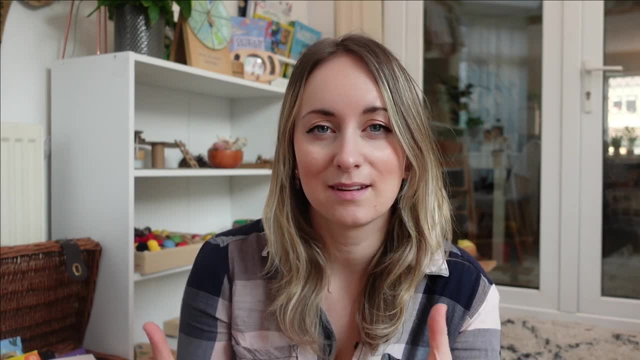 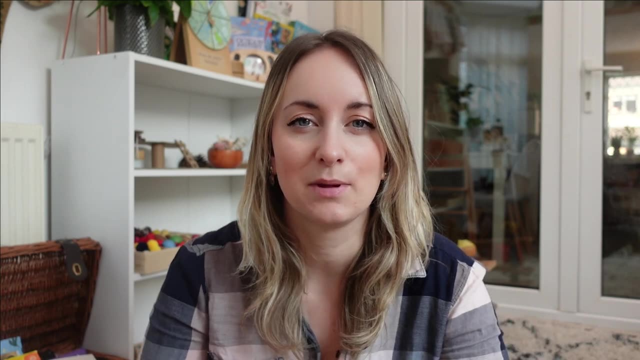 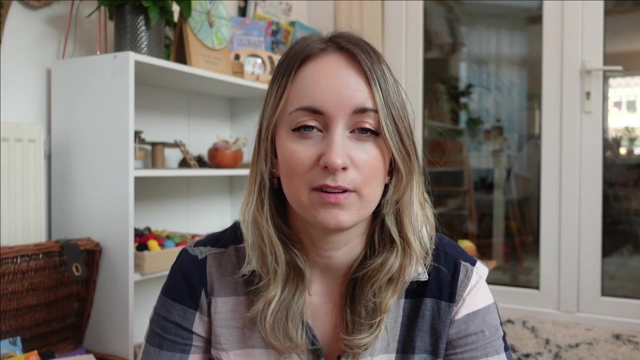 can transport them, move them around, make patterns. And this is the beauty of open ended materials is they serve no real purpose. There's no particular way that they need to be used And children are just free to, to play with them in whatever way, kind of they want to, whatever takes. 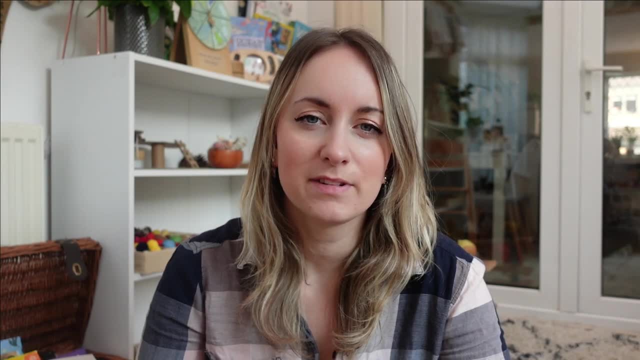 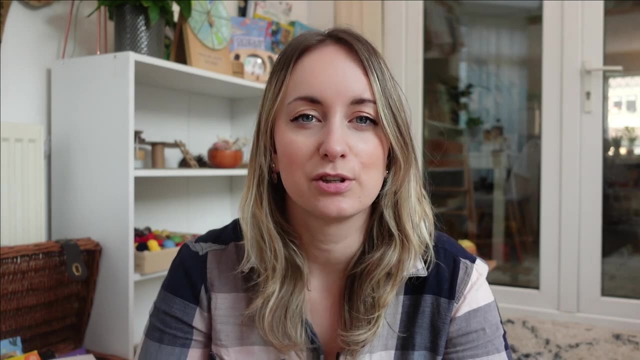 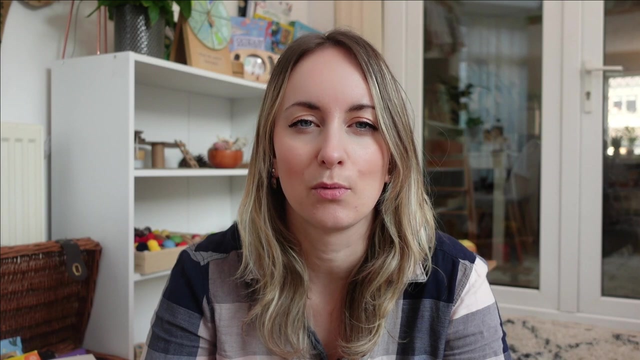 their fancy really. So, yeah, an invitation to play usually includes lots of loose parts, lots of open ended materials, So children can kind of go to it and think, Okay, what can I do with this? You know this is interesting. How can I explore this more? So yeah, an invitation to play can be anything. 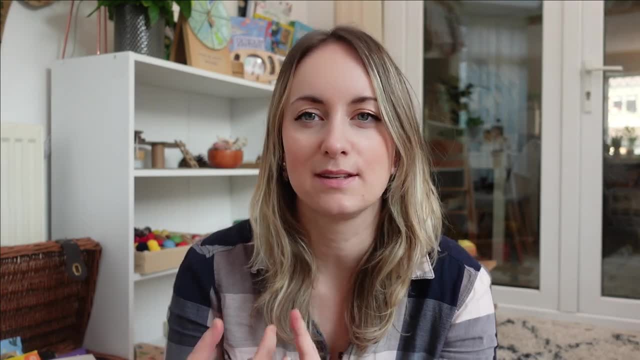 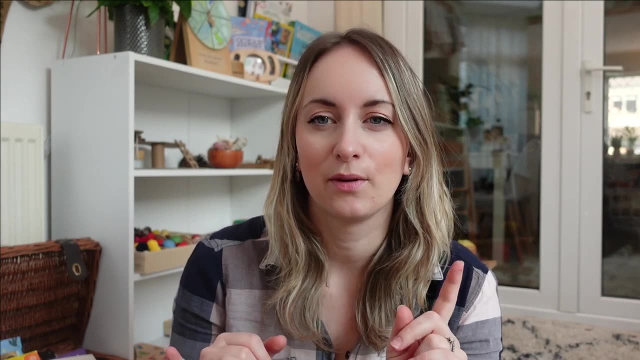 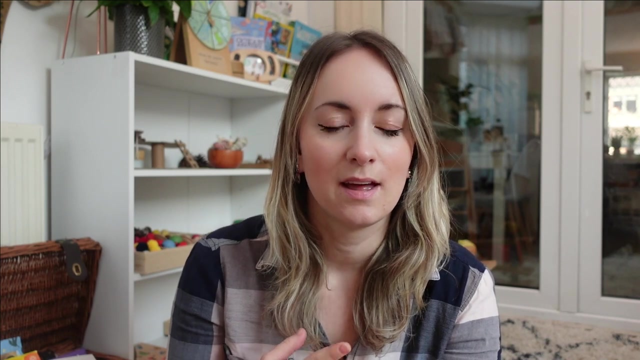 really It can be themed around a particular interest. So if your child's into whales, you could do a wave themed one. You can do ocean themes. you can do something to do with counting if they're really interested in counting at that time, And you can incorporate the alphabet and literacy. you can centre it around one of. 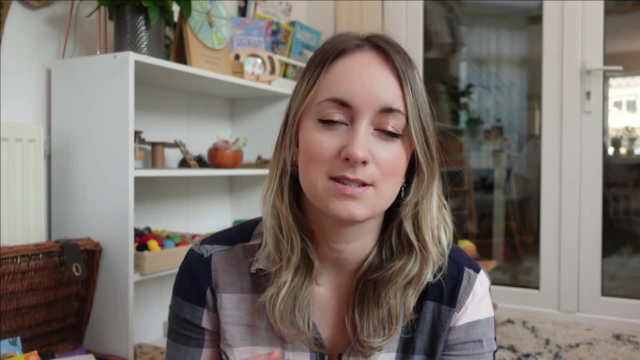 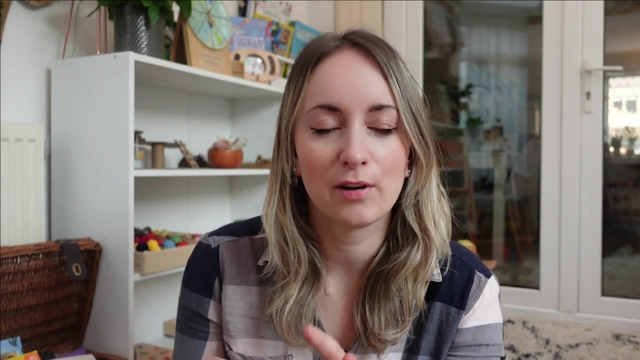 their favourite books, And so I've done invitations to play around. the time you came to tea, which was a real favourite for a long time, So we had lots of different setups with teacups and loads of different loose parts and different tea bags, you know, with different smells, So there's lots of ways that you can use your. 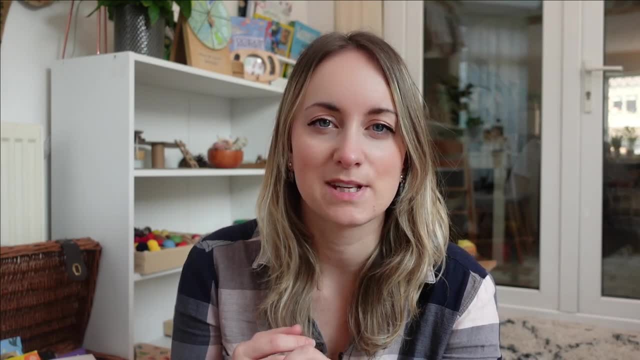 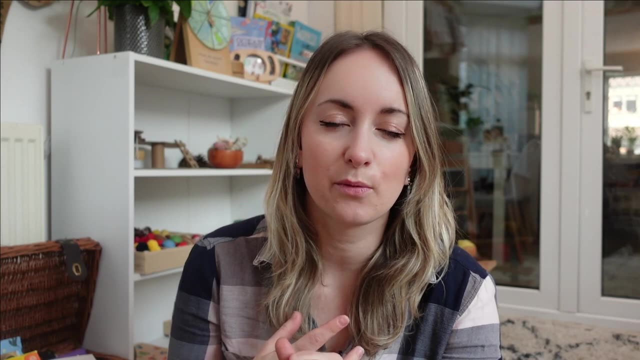 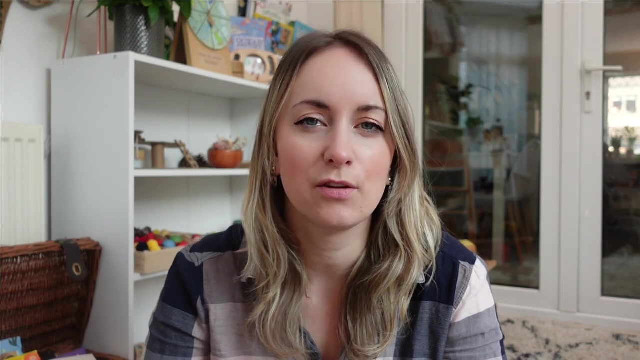 imagination to come up with just an interesting invitation, And you can do ones to talk about different animals, dinosaurs, you know. whatever your child is interested in, you can centre their invitation around that interest and you've got more chance of them being engaged in it. if it is an 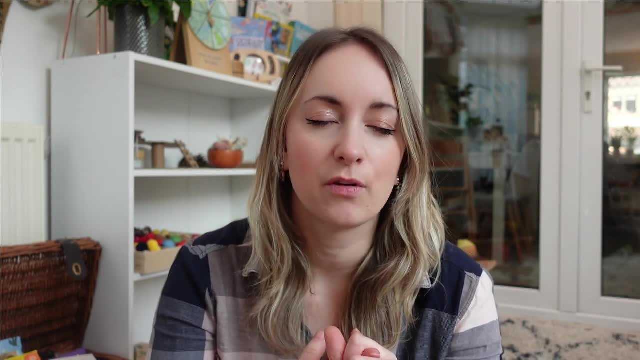 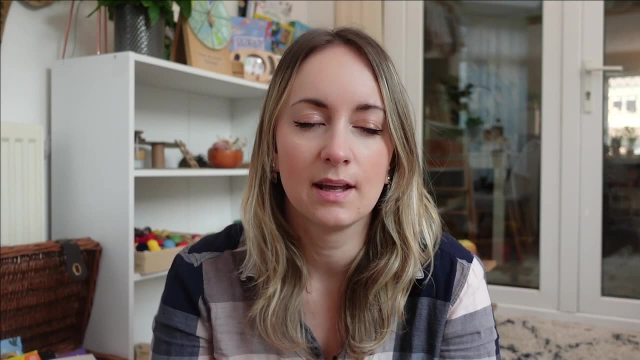 interest of theirs, And then you can do a little bit of a theme. You know, if you've got someone who loves transporting, you can do lots of loose parts, maybe some little boxes or bags for them to move things around in. So yeah, it's all about observing the child, seeing what they're interested in. 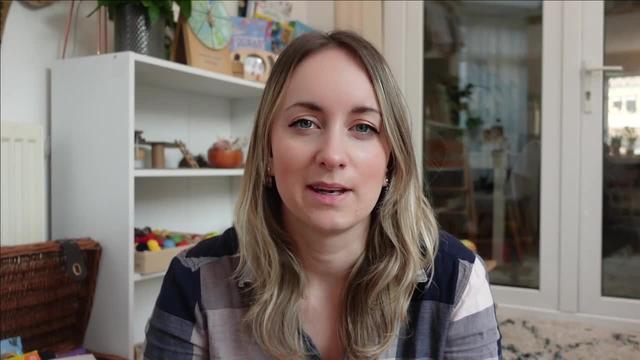 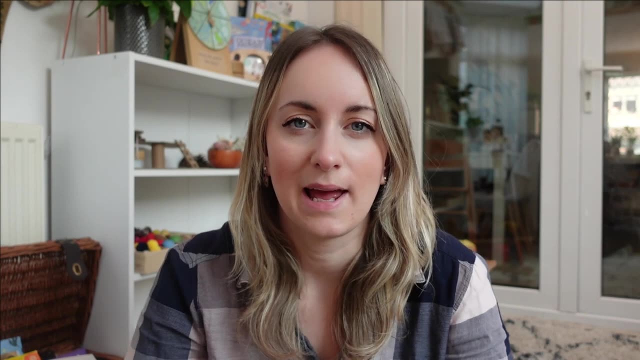 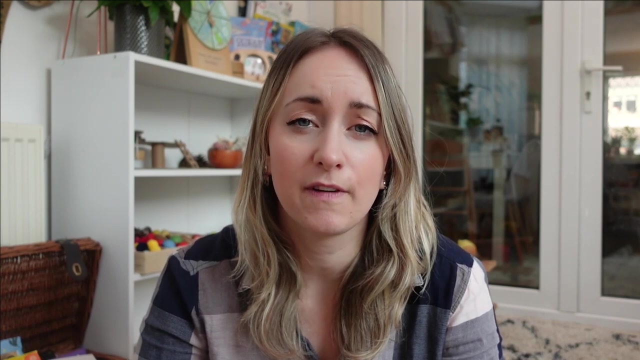 and just kind of putting something out that's gonna please them and engage them really. So, yeah, I'm going to share with you some really simple invitations to play. I've got four different ones that we've done recently, over the last few months, And they've been the children's favourite. 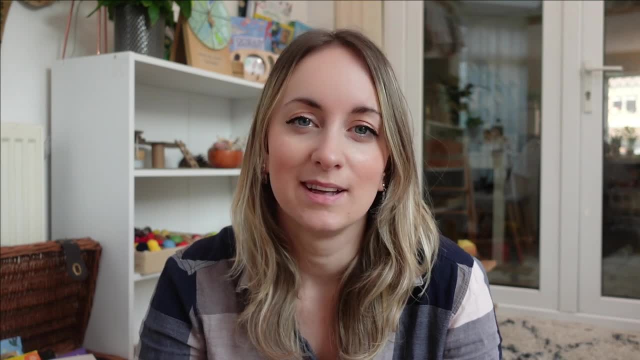 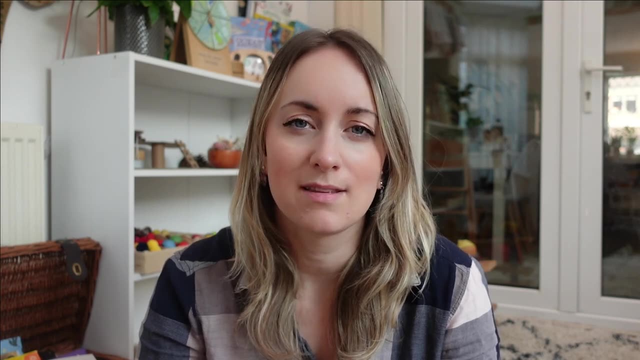 the most engaging. They're all really really fun to play with. They're really fun to play with, They're really engaging for them and my favourite as well to set up. But I don't want to give you anything too crazy or complicated. I always use really simple materials in my invitations. I just 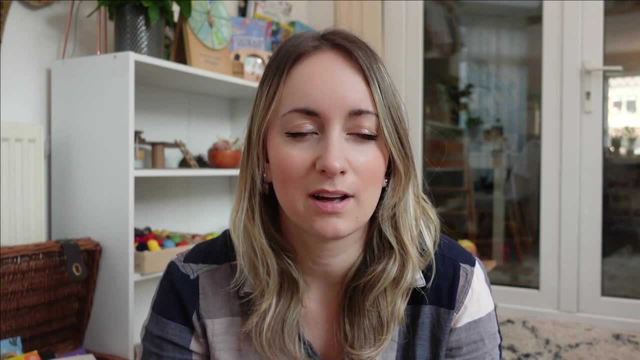 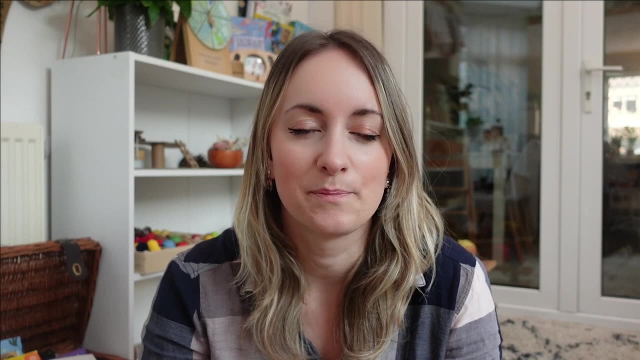 don't have time to make anything too crazy or intricate And I like things that are quick because the children, as soon as they go to it, you know if it's engaging for them it's destroyed anyway. You know they're moving it around. they're kind of 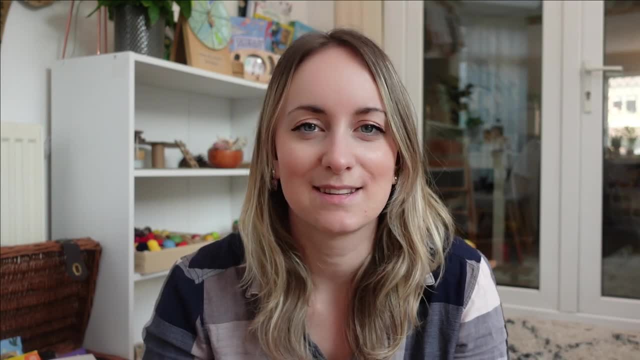 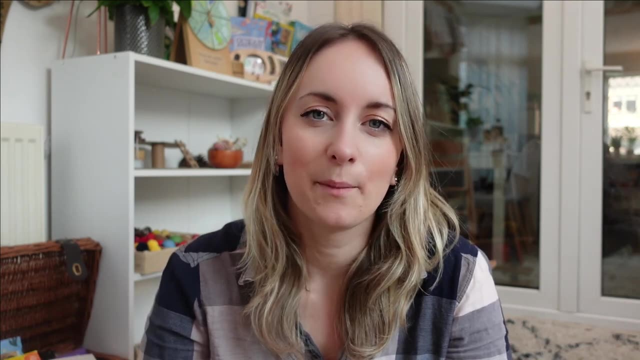 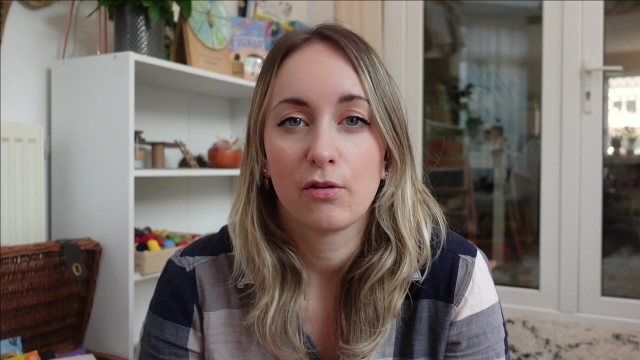 tipping things over and they're really getting into their play, And it's never a pretty sight afterwards, But that's what play is all about. So yeah, I'm going to share with you some ideas And hopefully there'll be things that you can kind of recreate in your own home, if you like the idea of. 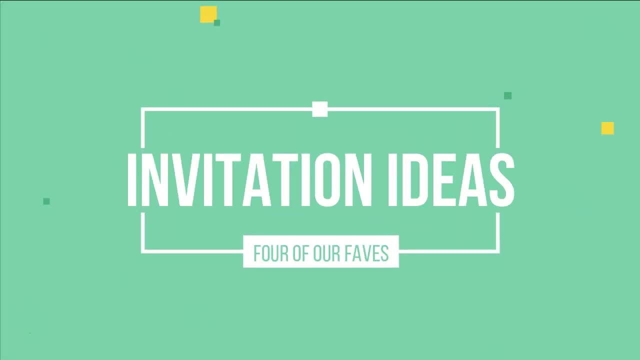 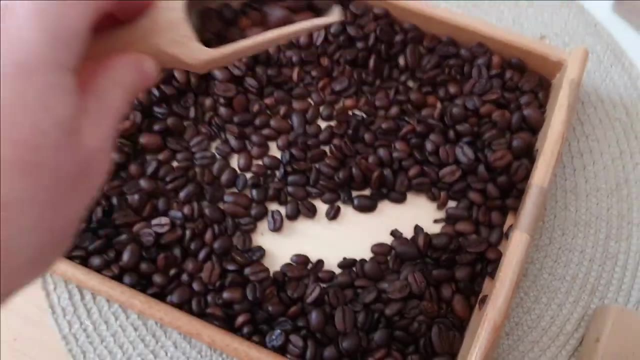 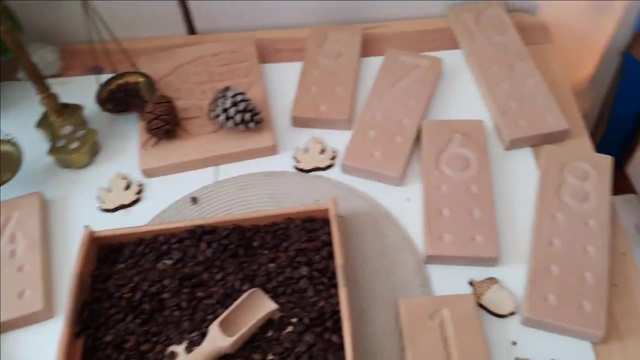 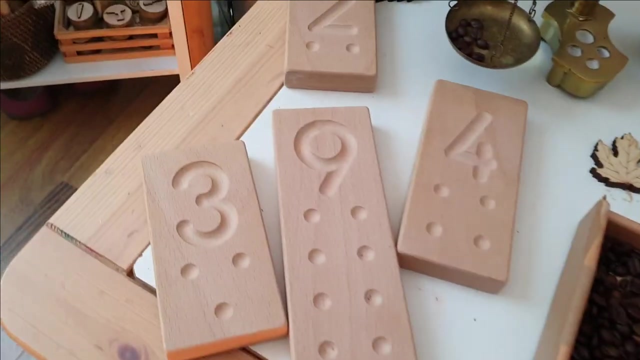 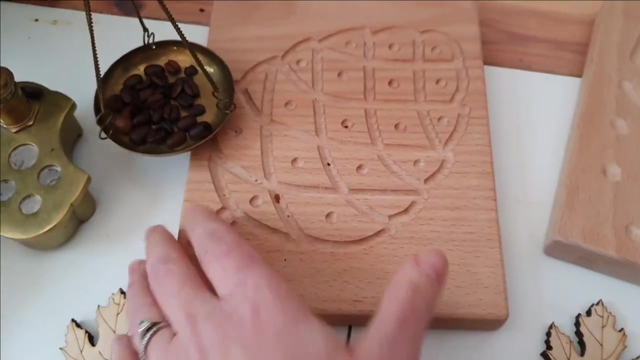 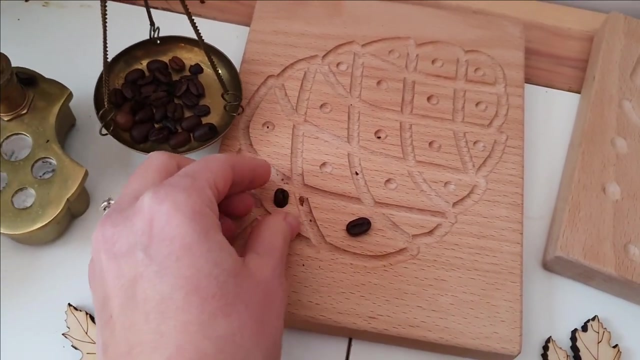 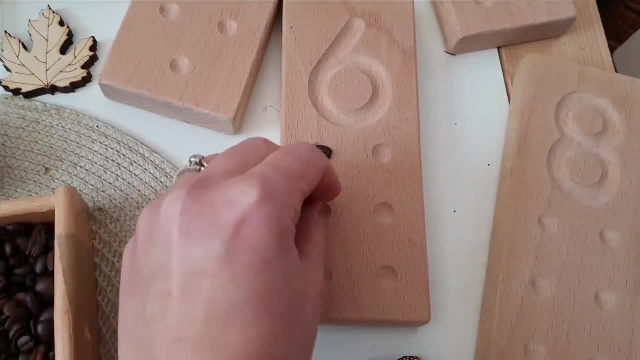 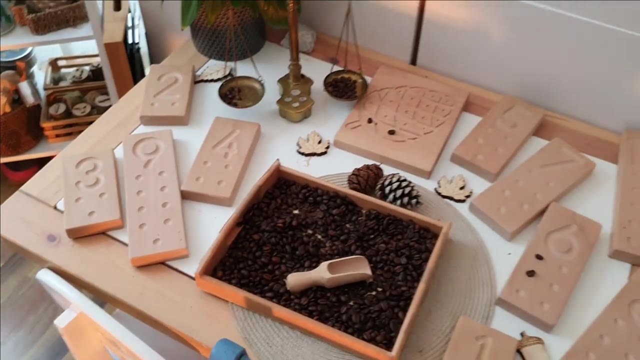 use And it's really really easy to use. And it's really really easy to use. And the number boards are actually counting boards but you can use them for so many things. So children can use them for number recognition and for tracing, But actually the coffee bean activity was one of my favourites. 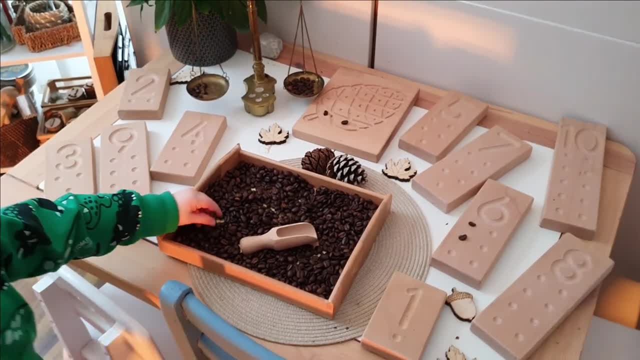 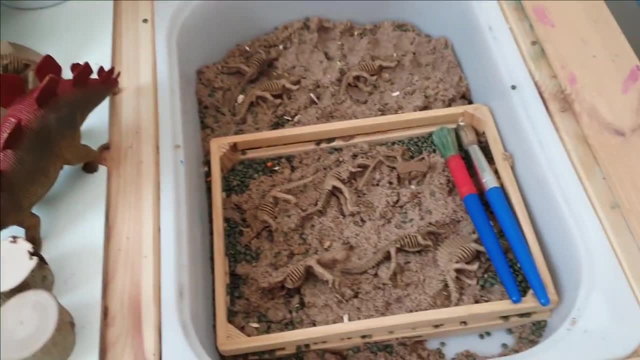 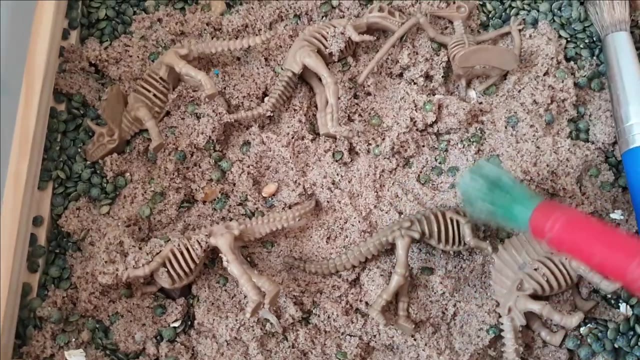 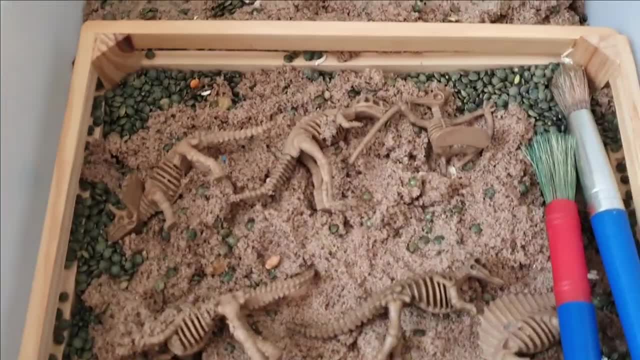 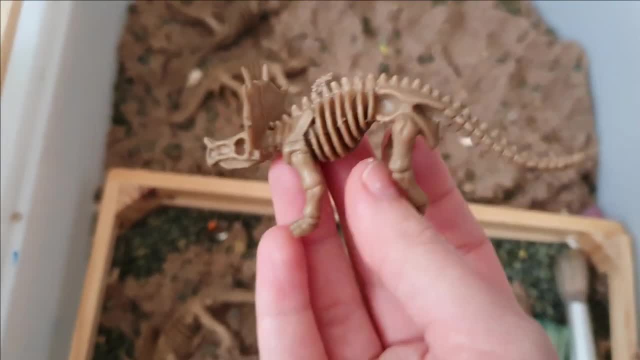 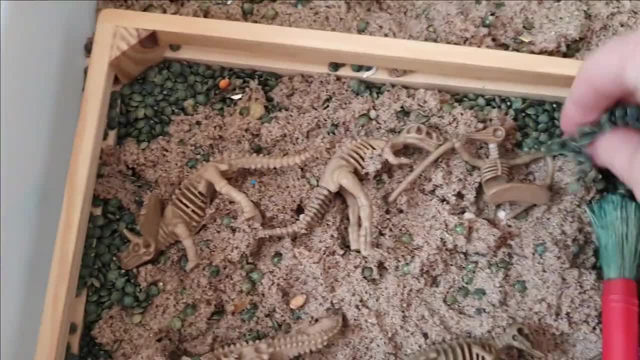 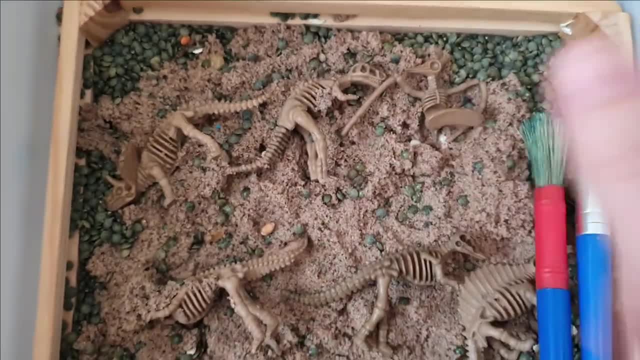 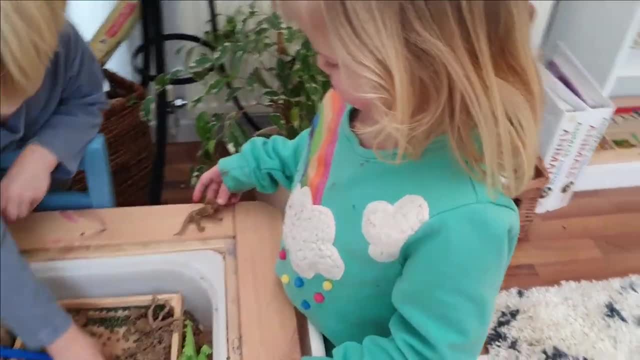 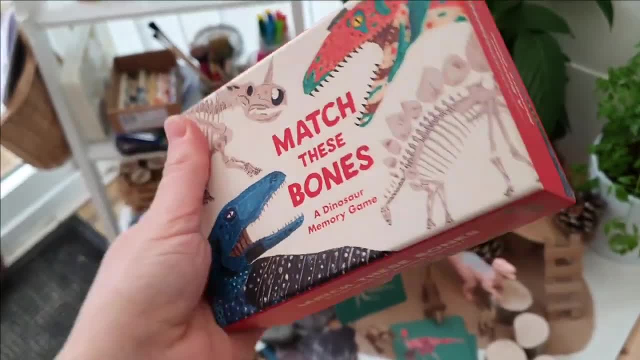 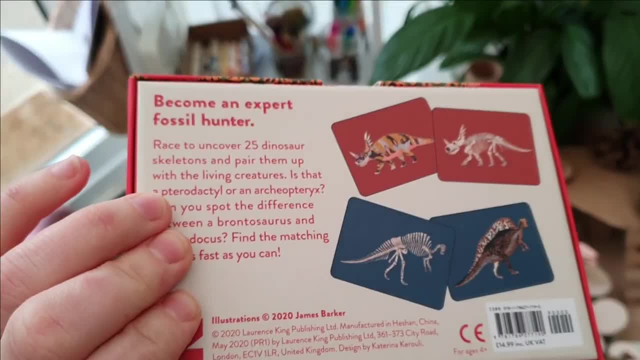 I absolutely love the smell. It went all the way through the house. I absolutely love the smell. It went all the way through the house. I absolutely love the smell. It went all the way through the house. dinosaurs- it's a little bit advanced for their age, i would say, but it's a really cool, um kind. 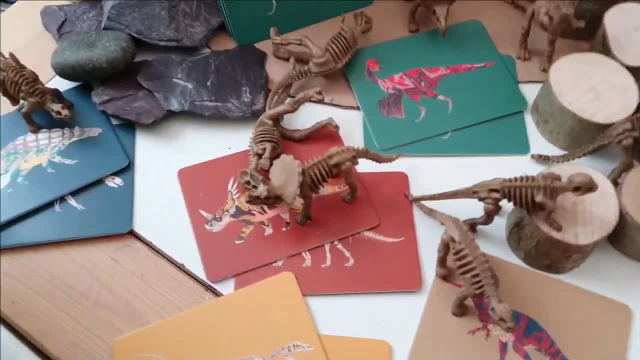 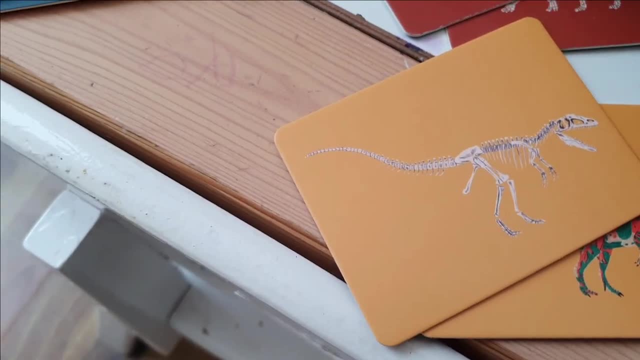 of introduction to go alongside the bones and they love looking at the pictures and trying to guess what dinosaur they are. so there's always variations you can do to kind of simplify it if you feel like an activity is a bit too advanced. but they really enjoyed him. 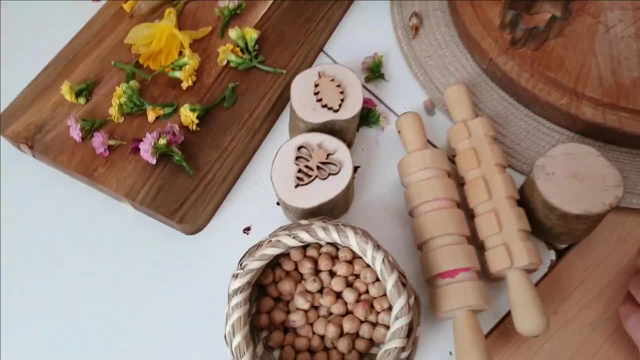 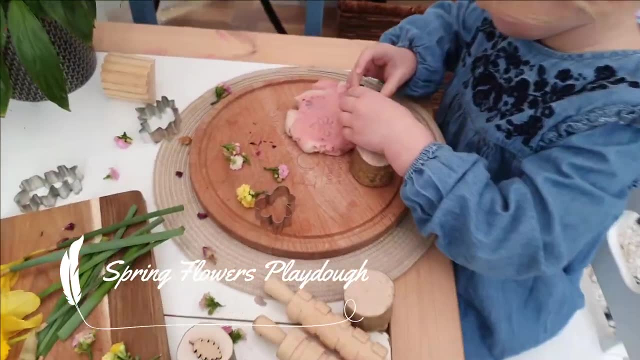 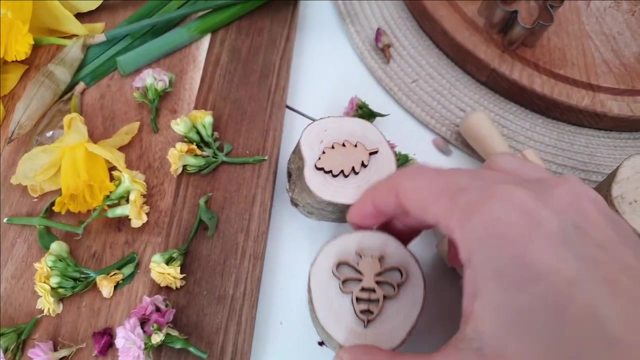 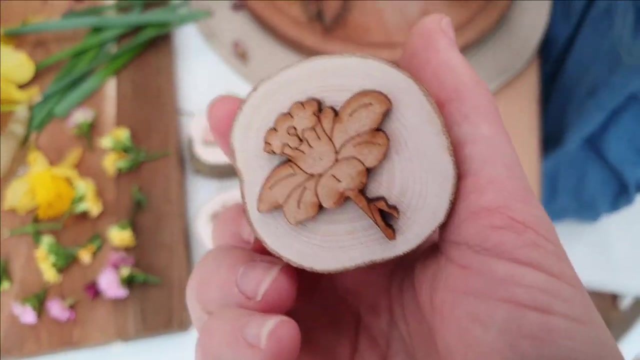 so these stampers here are actually part of my spring set. those who don't know, i have another business called the wild play nest where i make and sell sustainable play-doh stampers, all nature themed, using natural materials, and these i'm showing you now are part of my. 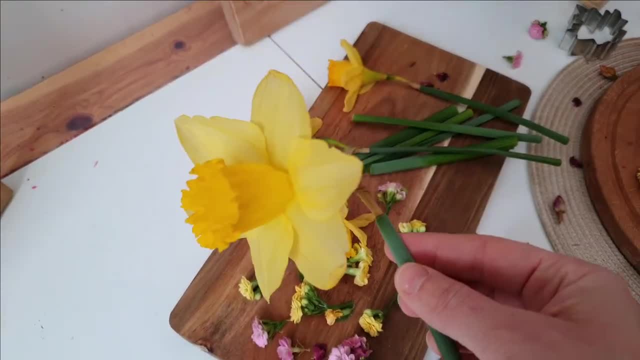 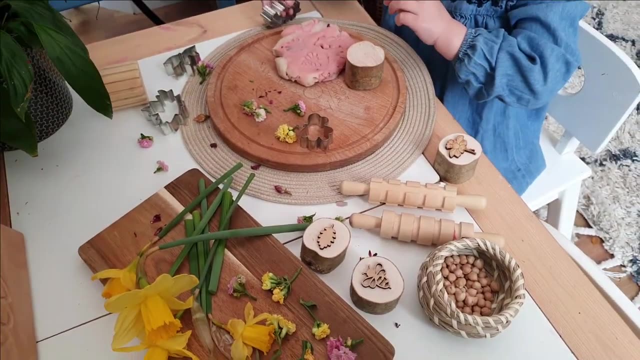 new stampers newly released spring set, which is a set of seven all spring themed stampers. I'll link my shop below so you can have a look. but this activity was really fun because I love any activity involving flowers. I just think they're so beautiful. they can be used in so many different ways, whether 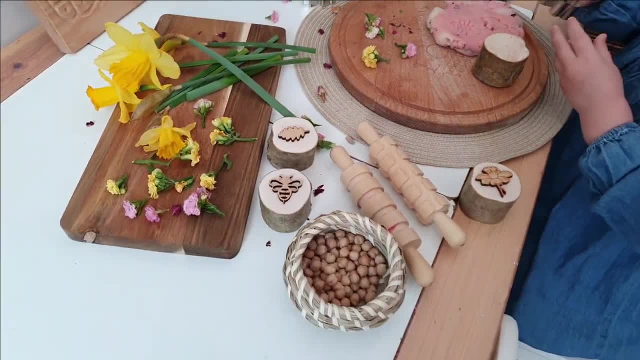 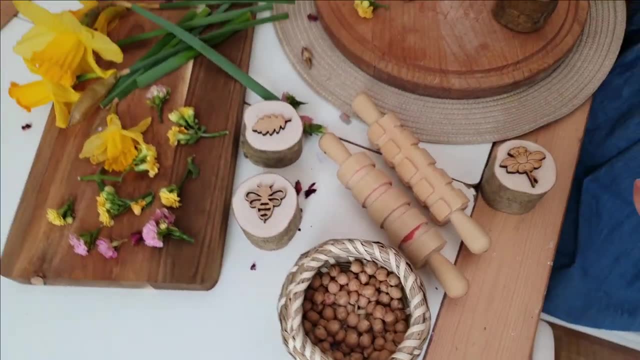 they're dried or fresh and you can kind of find them together when you're out on walks. so it's another way to kind of bring your child closer to nature. but I also added some chickpeas, which I usually do when we do play-doh, because they're really cool for kind of pressing in and making. 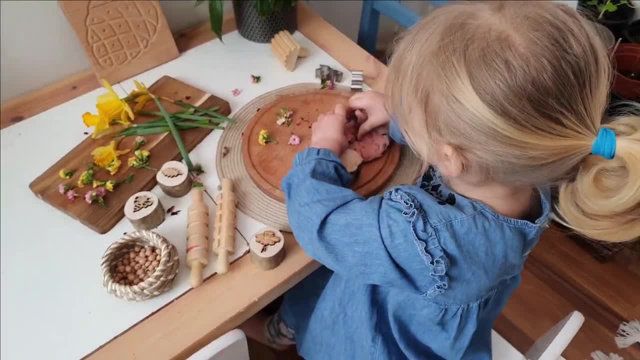 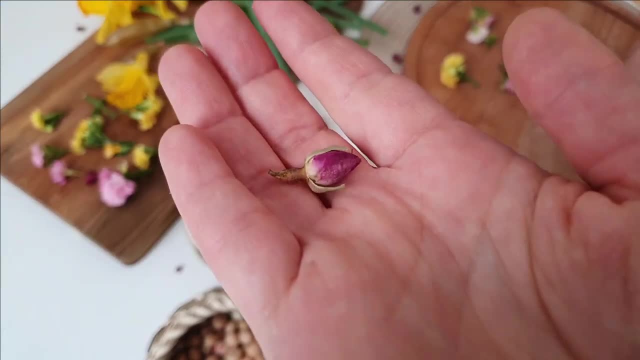 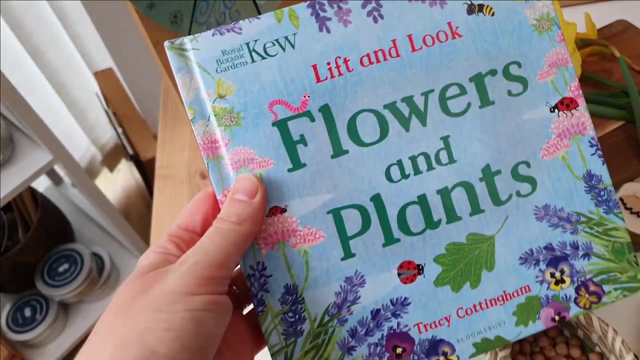 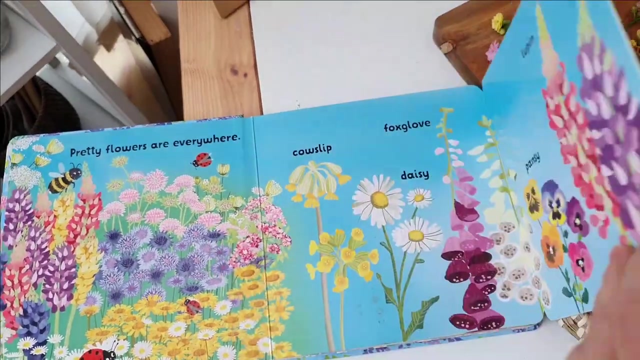 shapes and then some leaf cutters, or you can have flower cutters, but simple but really cool and fun. so I also added this flowers and plants book alongside the play, which is just an introduction to lots of different flowers and different names of the ones that we sometimes see when we're 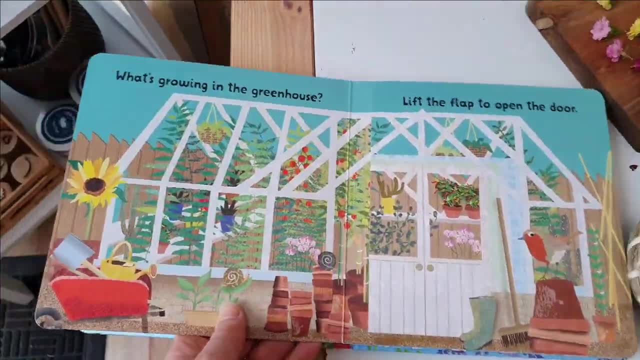 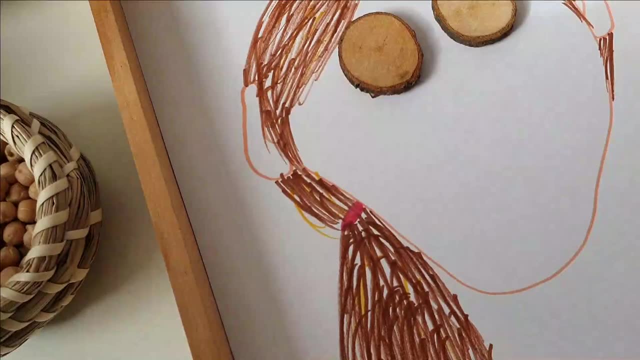 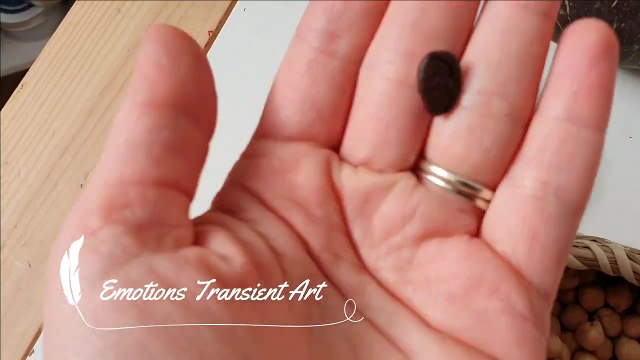 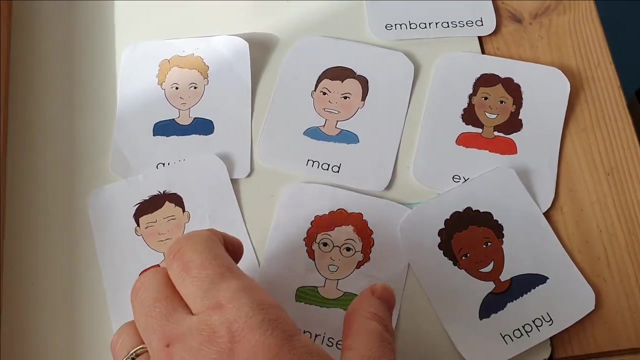 out in nature. but yeah, I always like to kind of add a book alongside because it just extends their learning. so I like to keep it simple, guys. I've used some of the same loose parts that we had in previous activities, so some grappa pieces, some chickpeas, some coffee beans, which we have an abundance of. 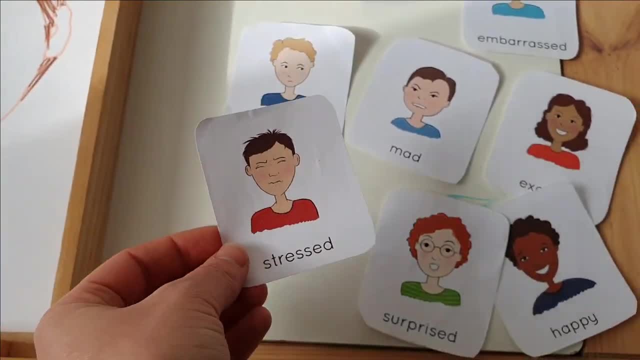 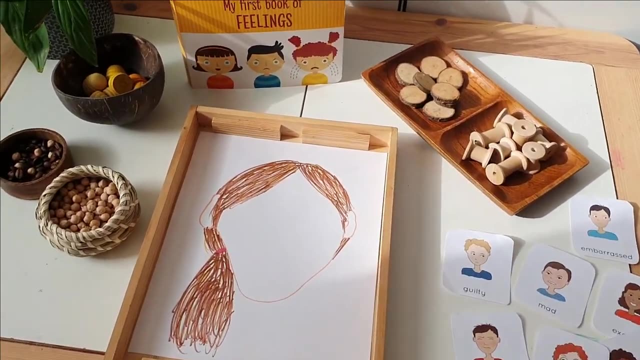 these are some cards that I printed off, which have all different types of emotions on, so there's new words there that they can explore, like embarrassed and stressed, which might not be words that or feelings that they'll be aware of yet, and then I drew this face on there. 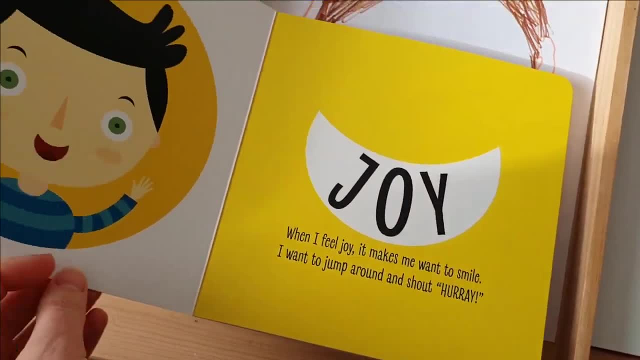 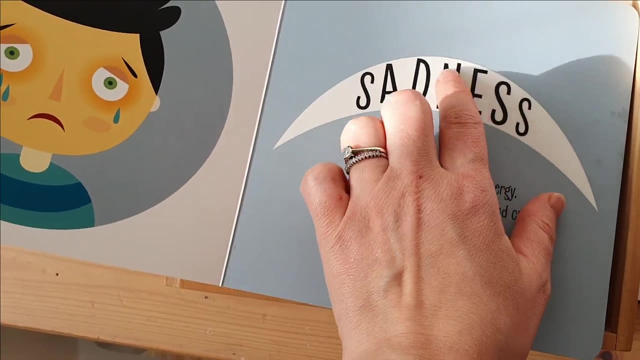 that they could fill in with all these different loose parts really to create those facial expressions and emotions. I put this book alongside because I always love to add a book and this is a really simple kind of explanation of of how you might feel if you're experiencing. 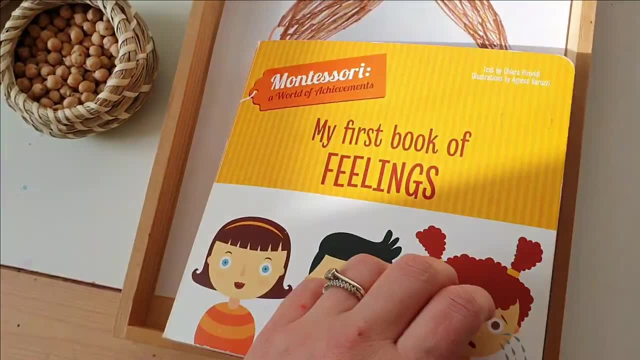 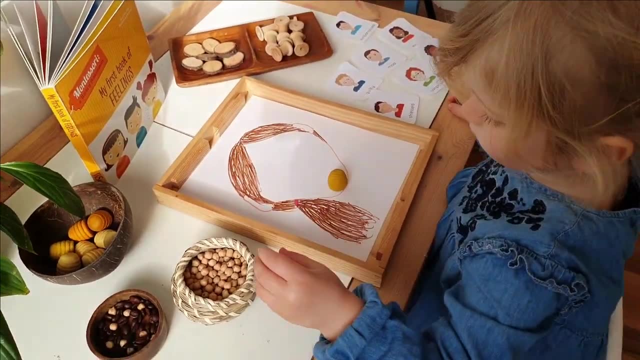 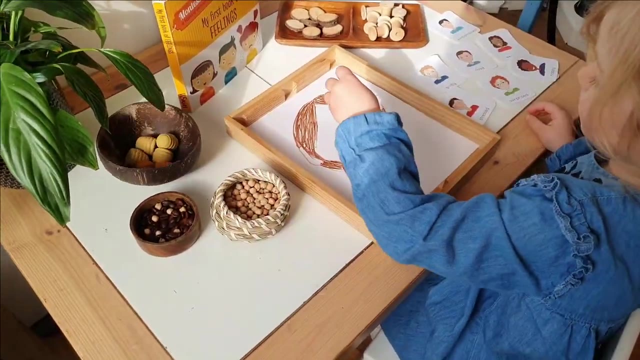 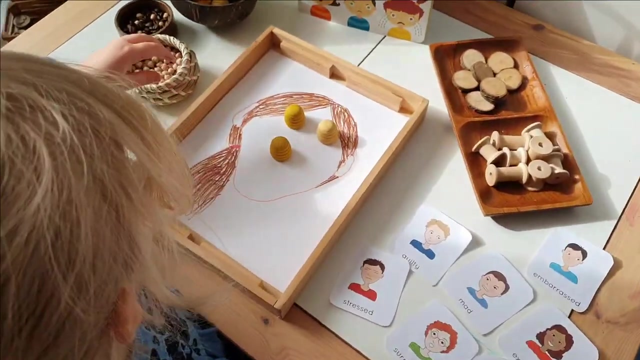 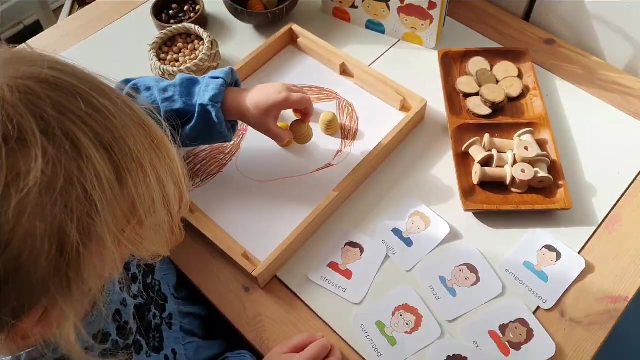 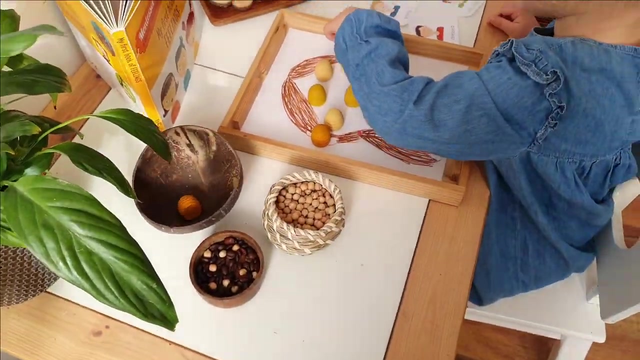 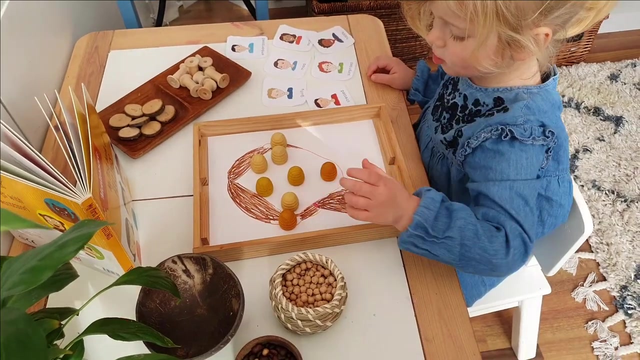 these different emotions and it gives little examples in there as well. those are eyes and a nose, yeah. cheeks, yeah, yeah, yeah, yeah, yeah, yeah, yeah, yes, yeah, yeah. but how are they feeling? what kind of, what kind of mouth are they going to have? yes, how do they feel? 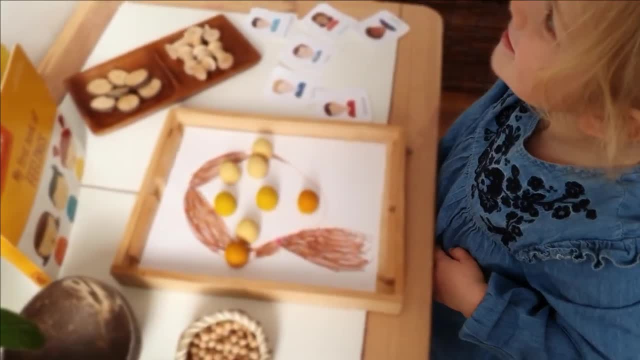 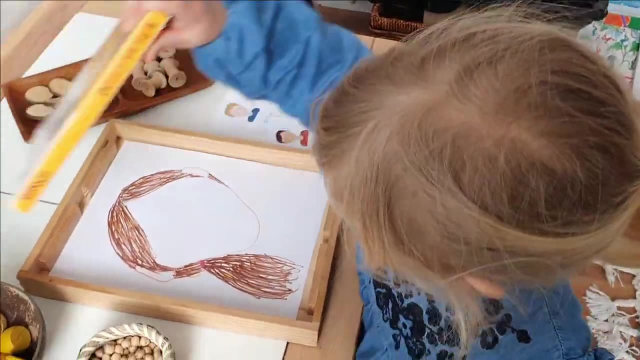 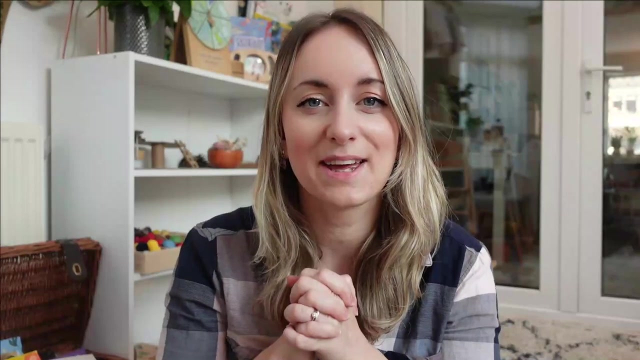 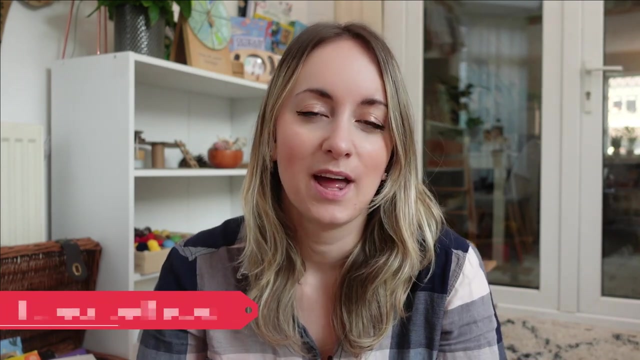 how do they feel me? they feel surprised. yes, yes, yes, yes. so thank you so much for watching. i really hope that was helpful and, as always, don't forget to subscribe if you're new to my channel. um and like. if you like um, and do let me know if there's any.